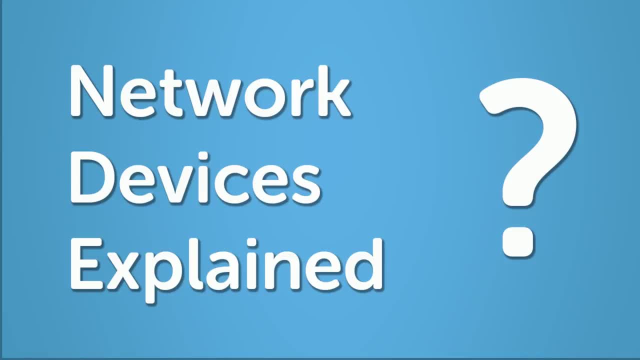 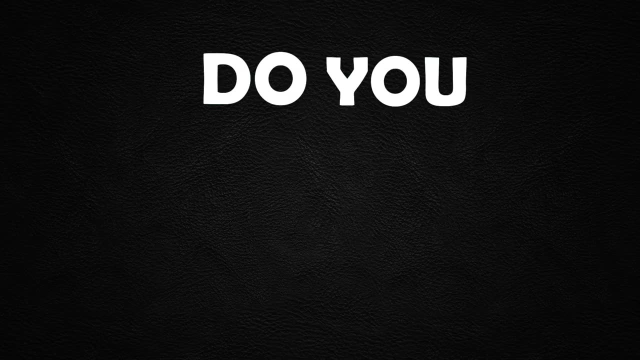 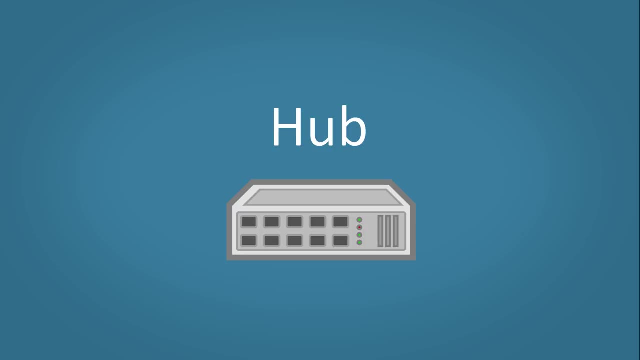 Welcome to CertBros. In this video we're going to be looking at four network devices. These are hubs, bridges, routers and switches. Okay, first we'll look at a simple hub. A hub's job is to connect devices in your network together. Let's see how it works. 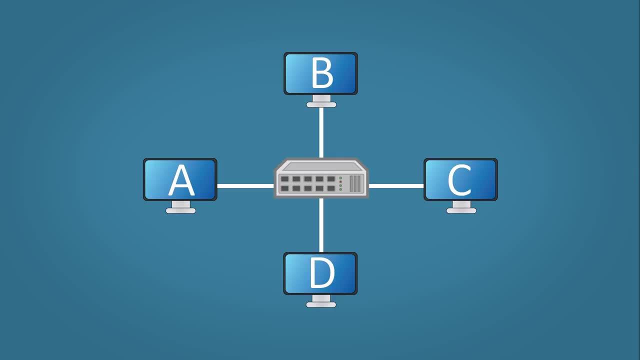 Let's say host A sends some data to host C. When a hub receives the data, it repeats it out of every port except the receiving one. Host C gets the data, but so does host B and D, so they simply discard it. 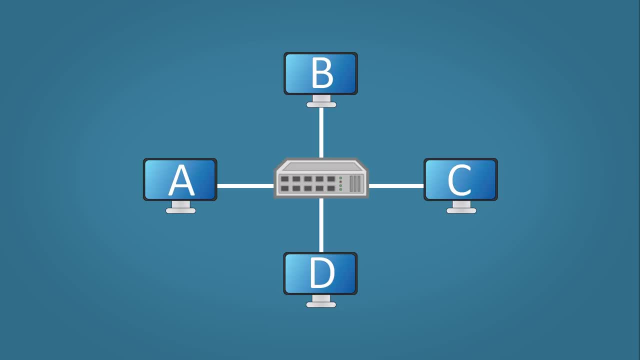 The hub has many downfalls. It wastes bandwidth, as we've seen when host B and D receive unwanted data. A hub uses a single connection, uses something called half-duplex, which means it can't send and receive data at the same time. 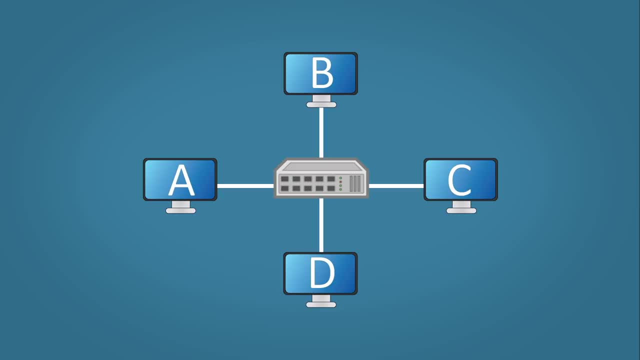 without causing a data collision. This would cause your data to become corrupt and need to be sent again. So, in overview, a hub is a layer 1 device, meaning it has no knowledge of addresses. All it does is repeat any data it receives. They have one collision domain and uses half-duplex. This means 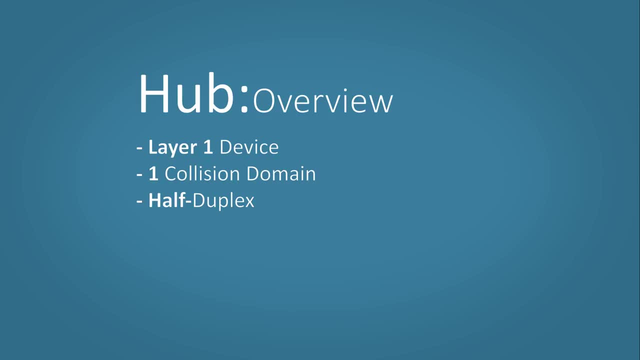 it can't receive data and receive data at the same time. They waste bandwidth by sending data to hosts unnecessarily. It has security risks because all the hosts receive everyone's data. A malicious user could steal this. Hubs are old technology. They have now been replaced by switches. 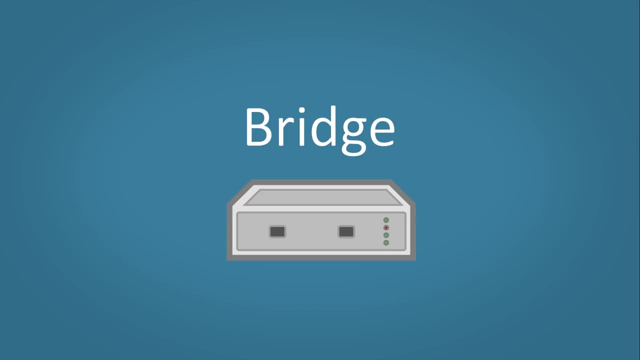 which we will take a look at shortly. Bridges were introduced to combat some of the shortcomings of hubs. They're used to segment networks into smaller sections. When data reaches the bridge, it decides whether or not to forward the data. It does this by looking at the destination and 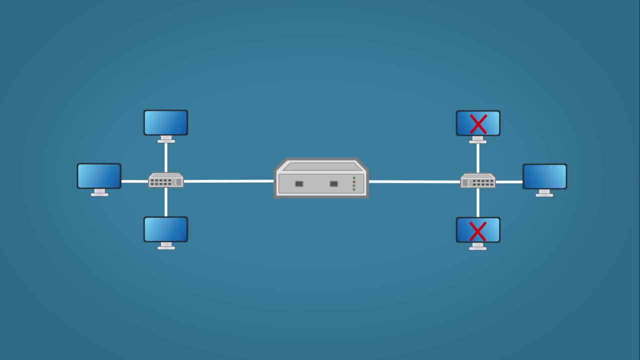 source MAC address. Every time the bridge receives data, it learns the source address, looks at the destination address and decides to send the data or discard the data. We will look at this process in more depth when we discuss switches next, as it uses a similar. 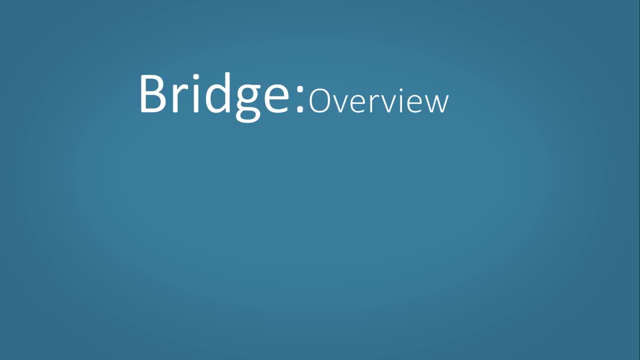 process. So a bridge is a layer 2 device. This means it can understand and learn MAC addresses. It segments LANs into smaller sections. It has two collision domains. This means data can be sent or received on each section of the network at the same time. 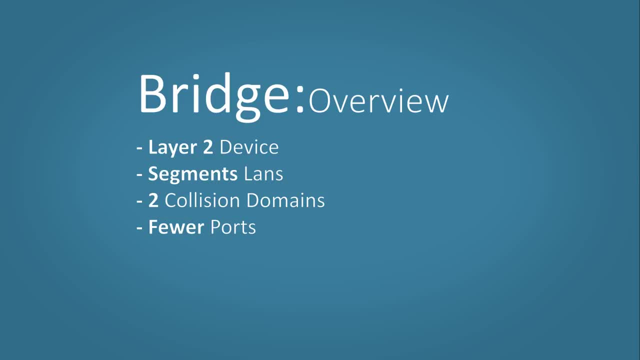 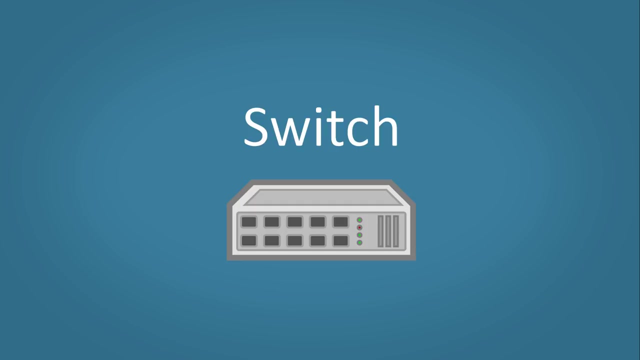 A bridge usually has two ports. Bridges are not used anymore. They have also been replaced by switches. Now let's take a look at switches. Think of a switch as a hub and bridge rolled into one. It connects the devices together, but it can also learn which ports connect to which hosts. Let's see how this works. 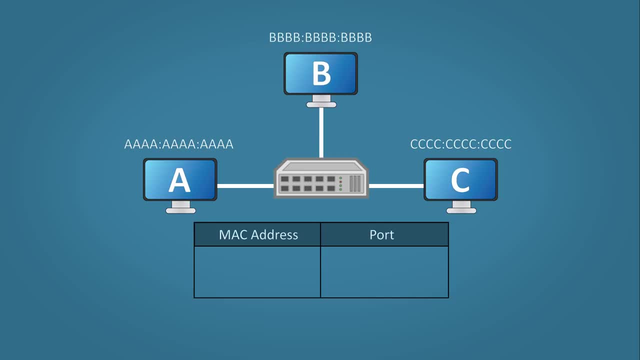 A switch has something called a MAC address table. This table will list each MAC address and which port it's connected to. In this example, host A will send some data to host C. The switch receives the data, but, as you can see, the MAC address table is empty. 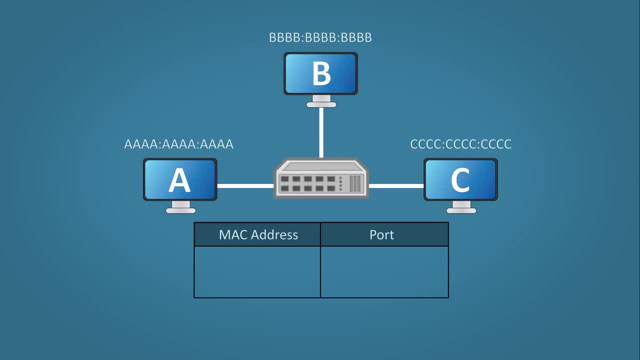 The switch in this case will forward the data out of each port, just like a hub. Unlike a hub, the switch now learns host A's MAC address can be reached on port 1.. When host C sends data back to host A, the switch knows exactly where to send the data. 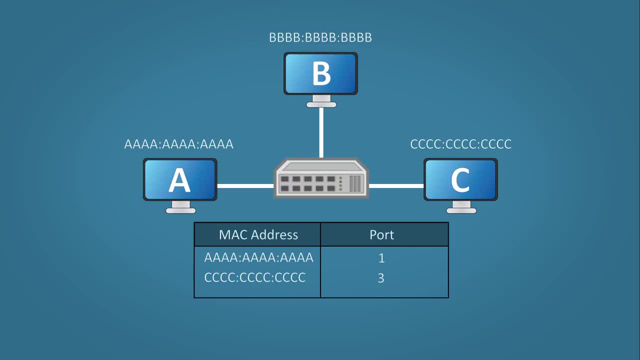 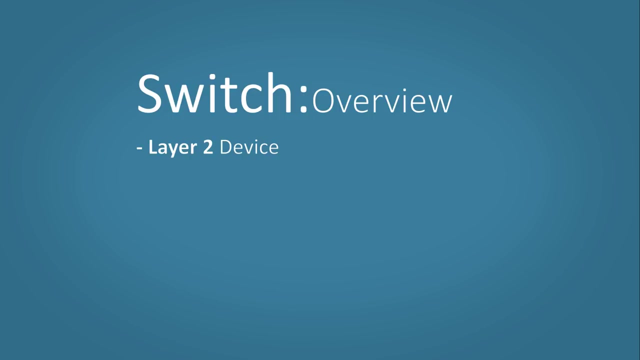 Now, if you notice, the switch has learned that host C's MAC address can be found on port 3.. Using this process very quickly, a switch can learn how to reach each host connected to it. Let's review. A switch is a layer 2 device. Like the bridge, it can learn MAC addresses, which are known as layer 2 addresses. 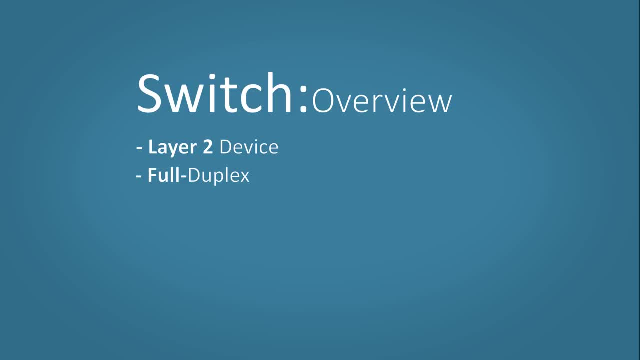 A switch can use full duplex, meaning it can send and receive data. This means each port has its own collision domain. This is a huge improvement over a hub, Because it can learn MAC addresses. a switch saves huge amounts of bandwidth And now because only the destination host is receiving the data. other hosts can't steal it. 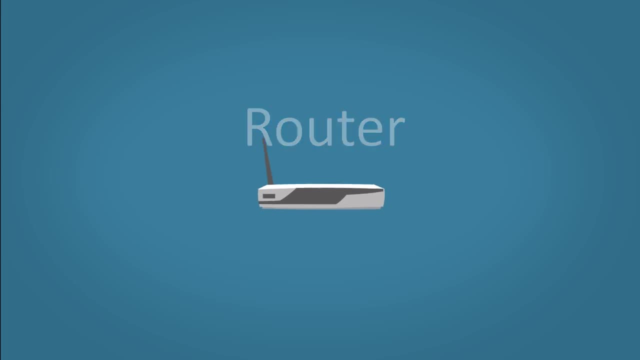 Routers. You can think of routers as the doorway out of your internal network and into the outside world. To understand what routers do, let's take a look at some examples. Let's take a familiar example. Let's say: this is your home computer, This is your switch and this is your router.